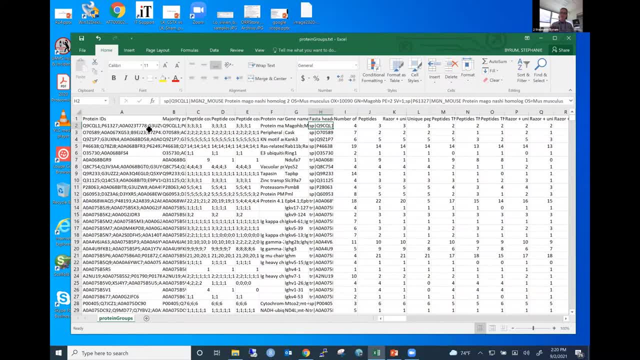 protein. we can actually add that protein sequence into the FASTA database as a new protein And then we can identify it in our database in our search results. But you have to know that information up front So you can customize those databases depending on if you have extra. 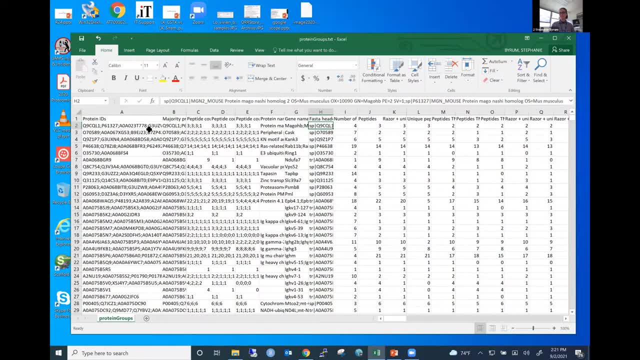 proteins or modified like mutated proteins And your sequence that you know about. we can make those changes before we do the database search and then we'll have it in our data at the end. So we have done that for several projects. The protein ID: this is where we have that issue with the shared peptides. So what it will do is: 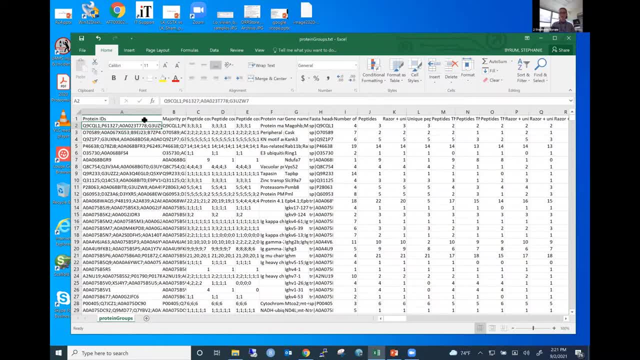 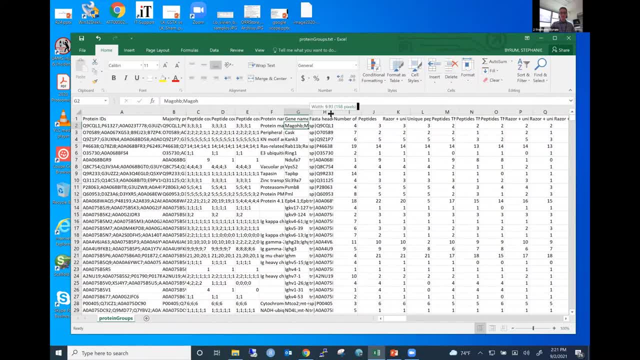 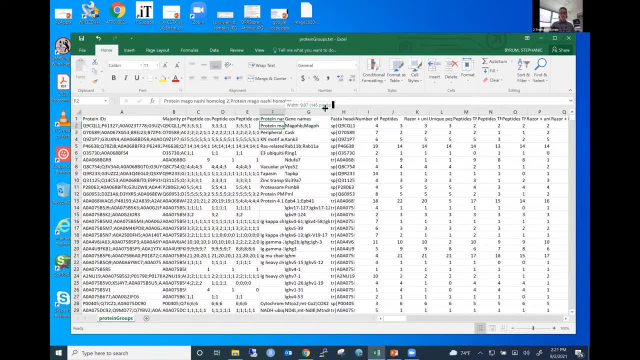 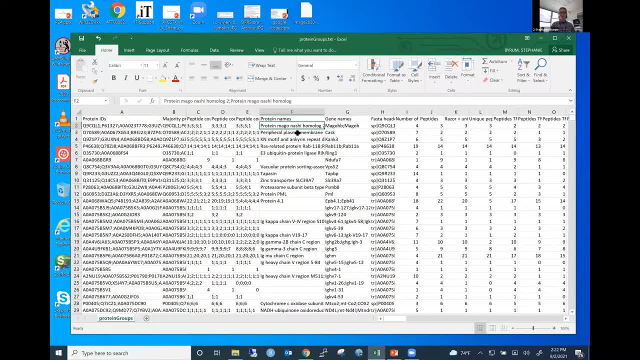 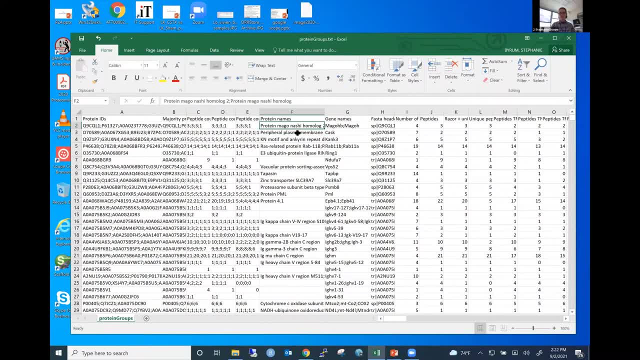 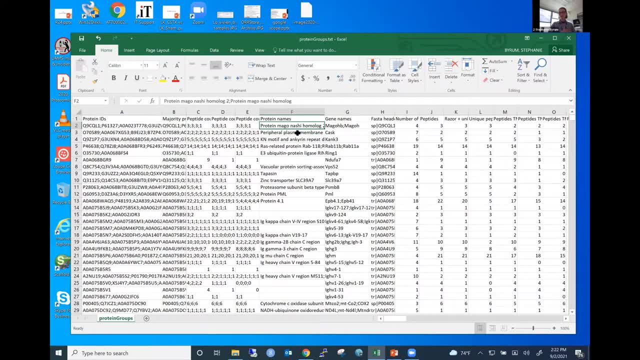 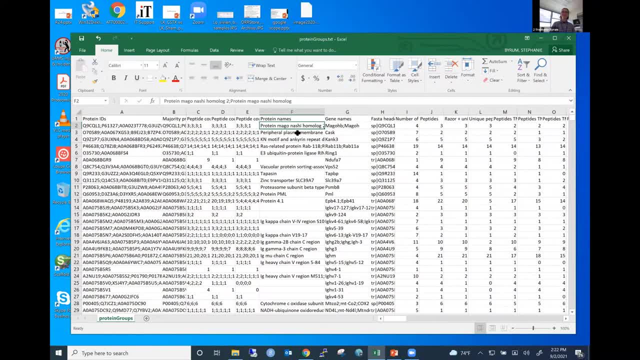 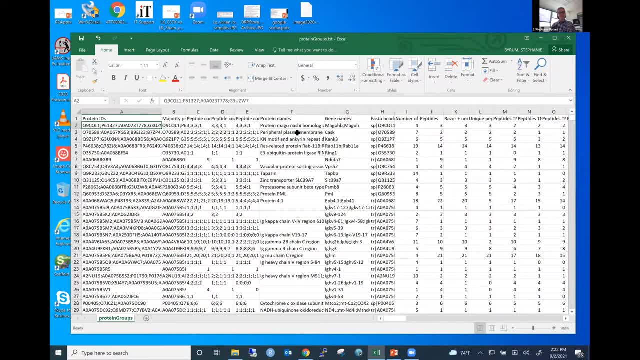 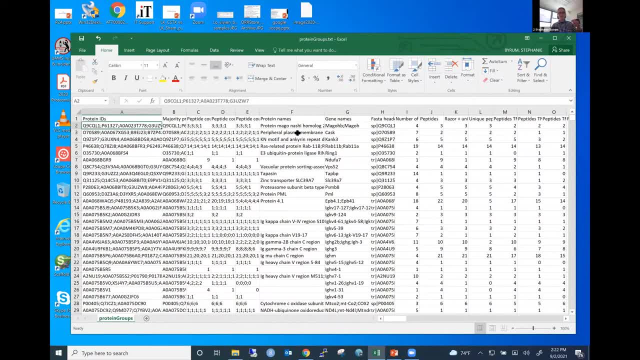 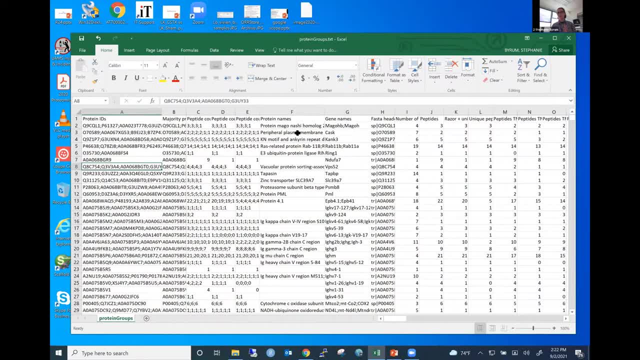 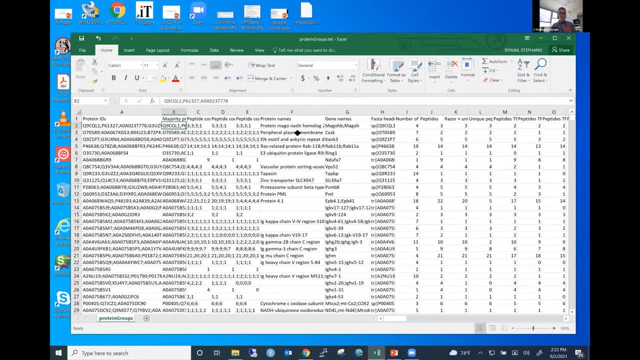 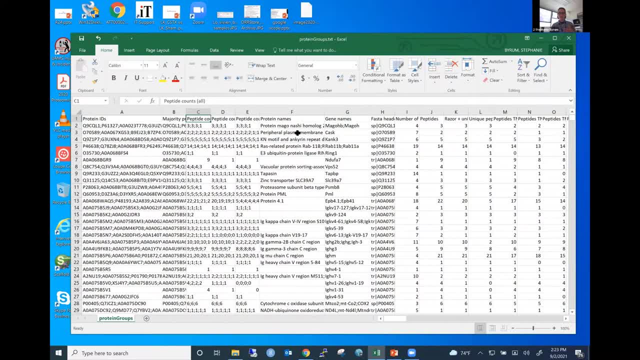 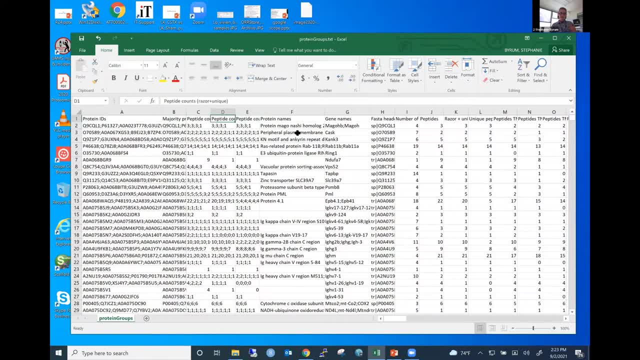 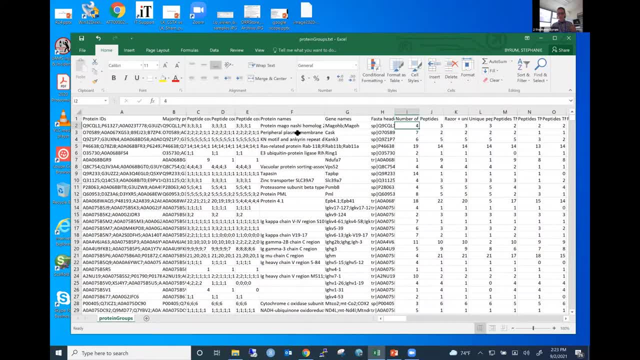 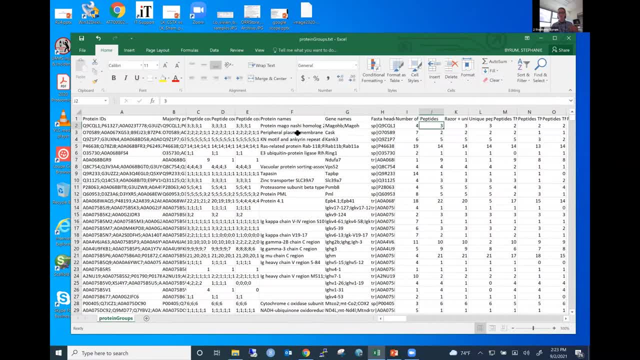 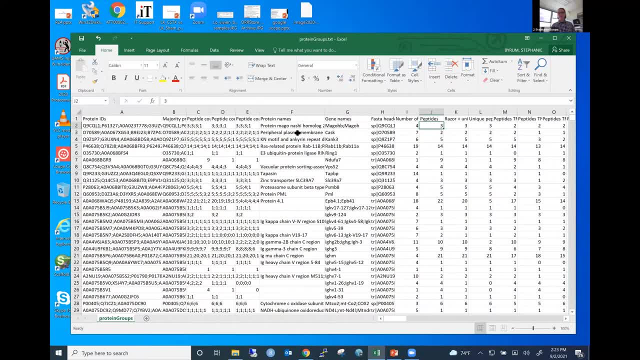 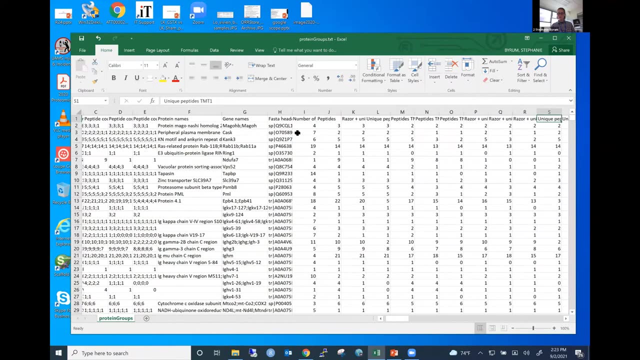 to that database search And then you can add that protein ID. but that can be dependent on also the size of the protein. So this one: we have 14 peptides that are related to that particular RAS protein. Then a lot of other count score metrics. 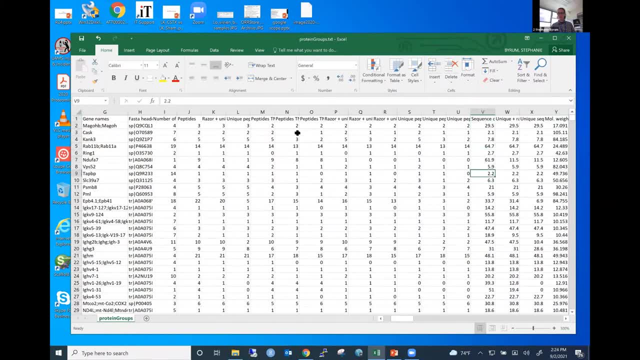 sequence coverage. how much of the sequence did we actually identify? percentage coverage: That's sometimes helpful to know that, like we just identified one peptide for this protein. so, depending on how strong of an identification that protein is, you're basing all your results on that one peptide instead of a higher percentage of the full protein. sequence coverage. 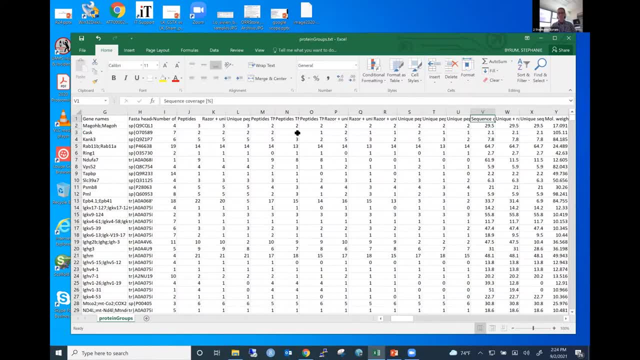 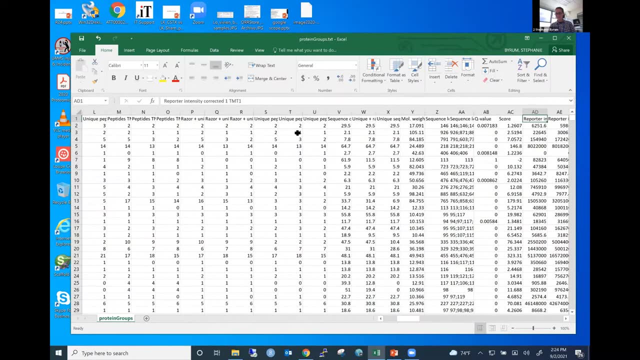 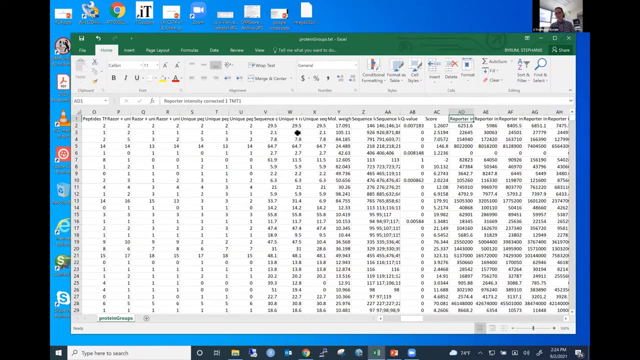 So those are some things that you can look into when you're really trying to investigate the analysis at a deeper level Scores. I have a slide deck that has some of the MaxQuant definitions, so I'll put that into the slack and then that way you'll. 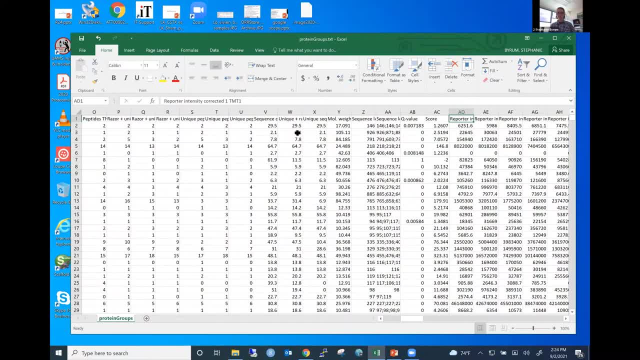 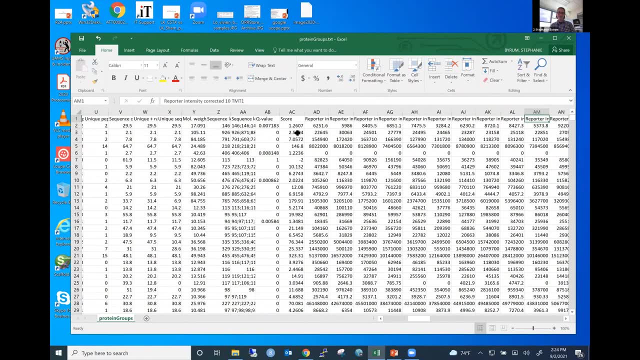 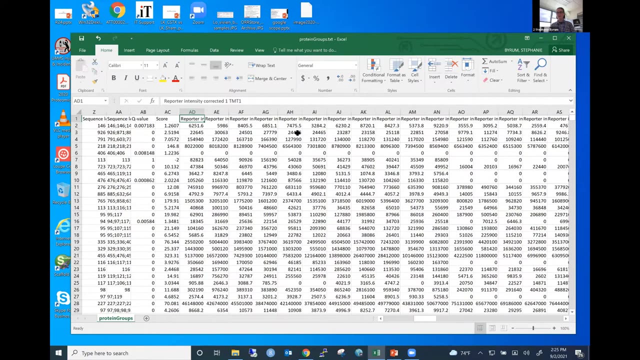 have the definitions of these different scores and stuff and you'll have those notations. What I wanted to point out here is the reporter intensity corrected channels. This is the columns that we were pulling out from the Protea Norm app to do the normalization on. So these are going to be those TMT reporter ions that are corrected for. 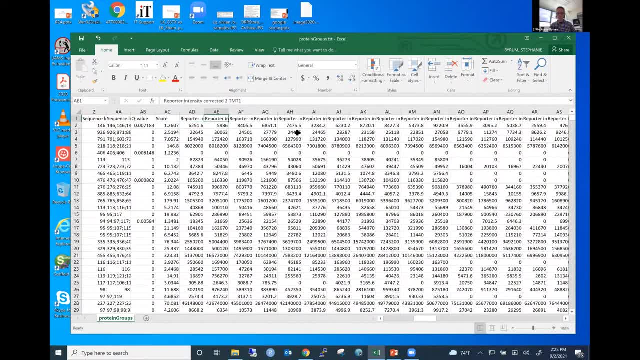 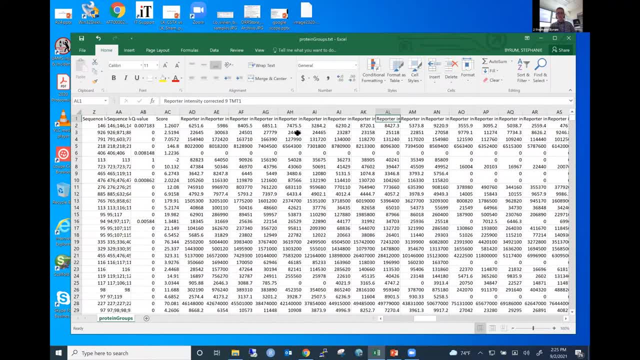 So you have the 1,, 2,, 3,, 4,, 5,, 6,, 7,, 8,, 9,, 10, 11, because those are going to be the 11 channels from the TMT multiplex And the only way you know what 1 is versus 11 is by that lot. 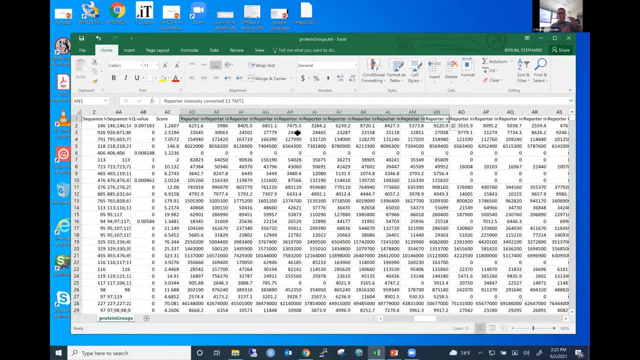 number description in the Thermo Fisher form. They have a pdf that says it's the 126 and 127 and 127c. All of those different mixings are in the order of 1 to 11 in the output of max quant. 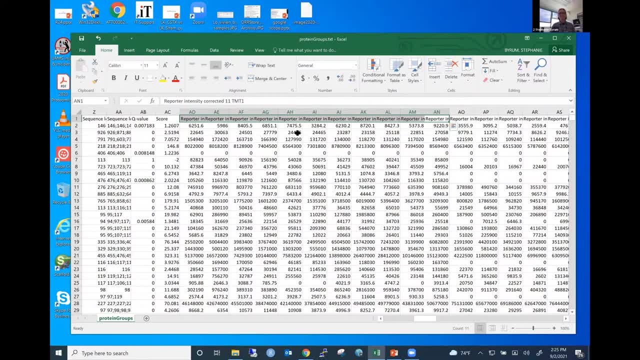 It doesn't tell you which actual isobaric label it is, It just orders them 1 to 11.. So we want to be careful when you're which the. the core helps take care of that. They do the sample labeling and we make sure that we have the right sample with the right number. 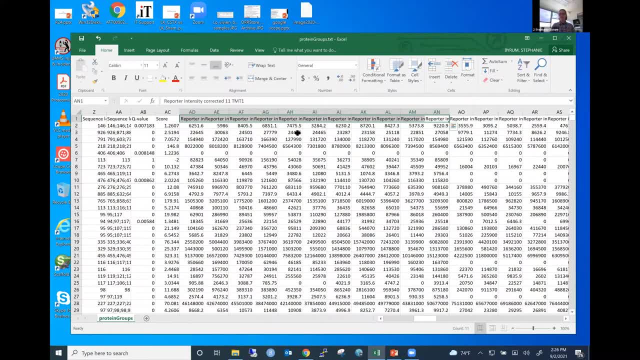 so that we can make sure that your sample names match up to the right information. There's a process in place for for keeping up with all of that information And then, if you'll see Here, I actually have this TMT1 tag versus the TMT2 tag. That's a. 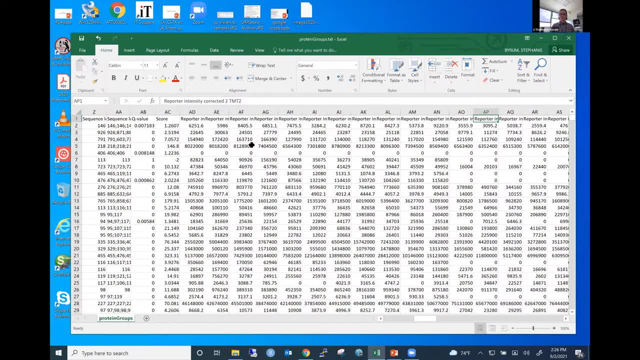 experimental design label that I gave the samples. in the database search of max quant You can set the label of your samples what you want them to be. So I just said TMT1 for the first batch, 2 for the second batch and 3 for the second batch. So it should be there Now. it points out that this: 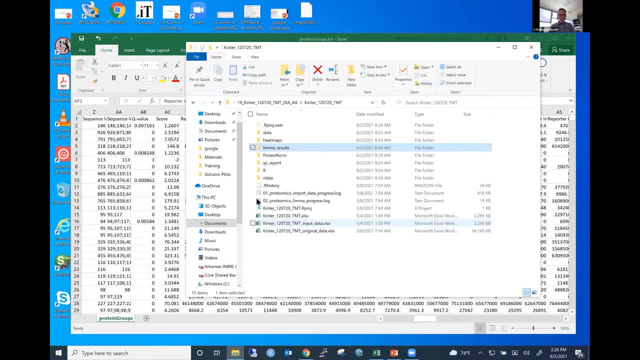 is just a process, So we want to explore each of those like in the classical world context. if we're trying to get this out of use for isobaric, the last 2 tables S arose Ng for 4.. And then we make a targets file, kind of like you do with genomic data. 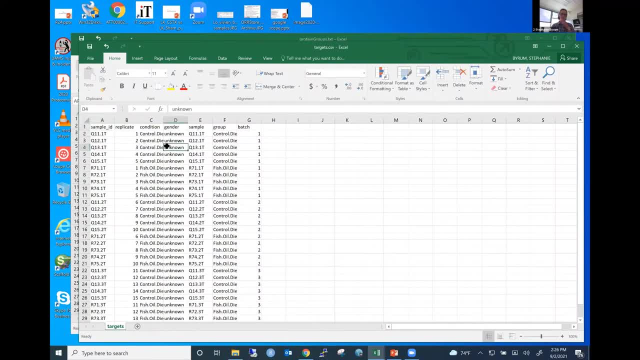 We just make the sample targets file. This one's a little different structure. Usually I have, like the reporter, ions in here and then which replicate it is with the information about it: Sample names, group names, batching. If they're paired samples we can put it at a column here for paired analyses. 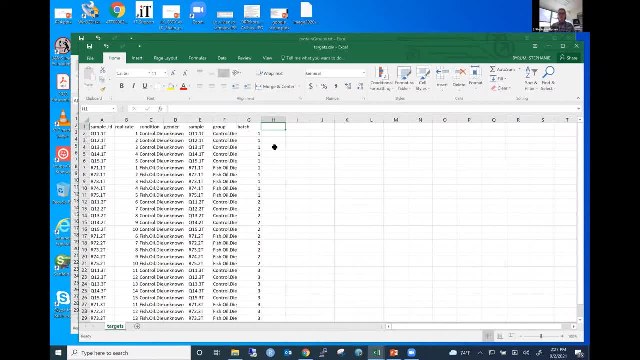 So all of those statistical questions that we want to ask up front, we're setting in this sample group targets type file. That way when we process our code we have it set up to where it can automatically detect if we need to do a batch correction or a paired analysis or not in the statistical design. 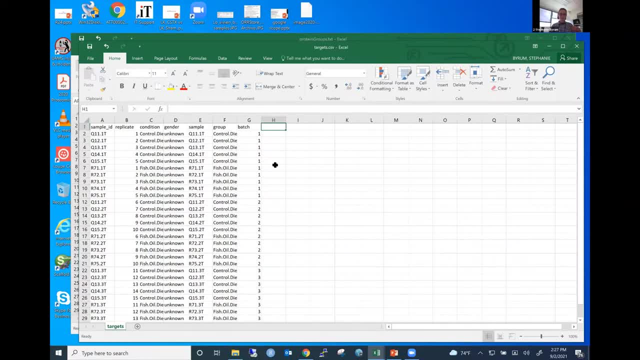 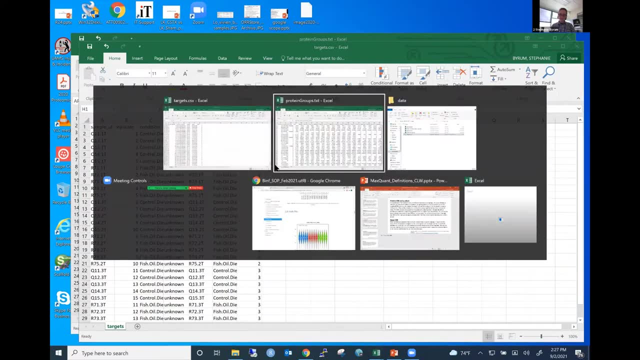 So we try to help ourselves out and be able to put the variables within this one file, And now I'm going to change the code every time. Every time we run a project. Let's see what else to in here. So these are going to be your raw values. 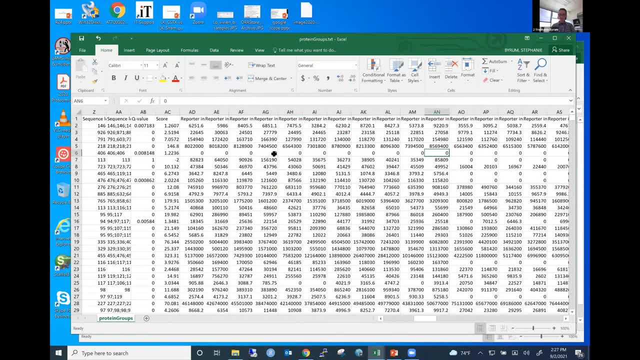 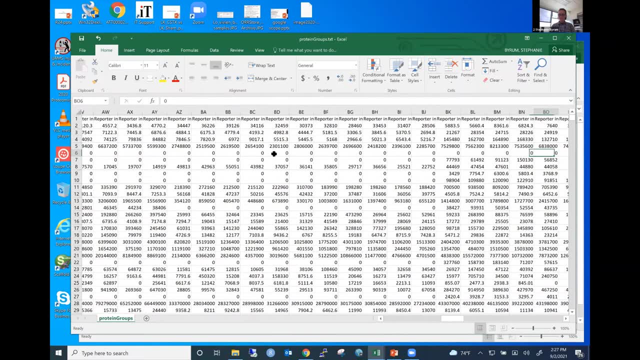 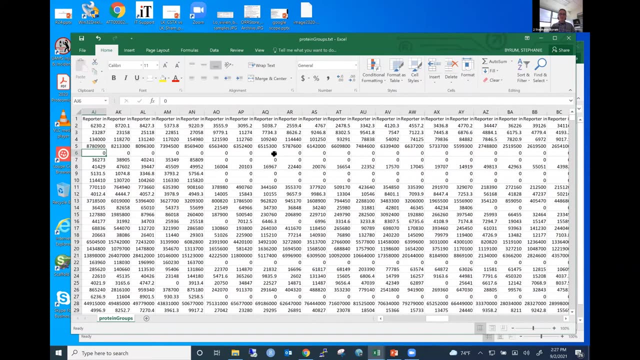 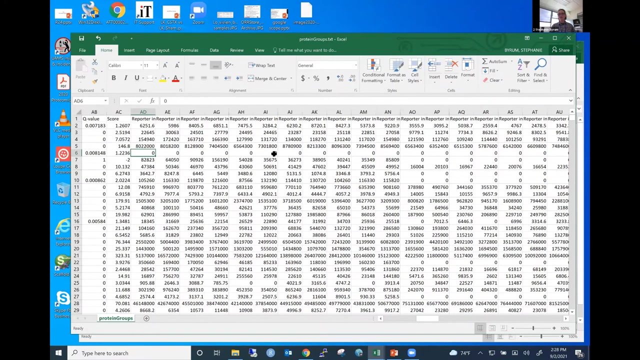 And you can already see, there's this missing set of intensities in those, all of those columns, So that particular protein had just enough of an MS spectra to be identified, but not enough for a quantitation. So we would actually Filter that out. if there's a zero across all samples, that gets filtered out of the analysis. 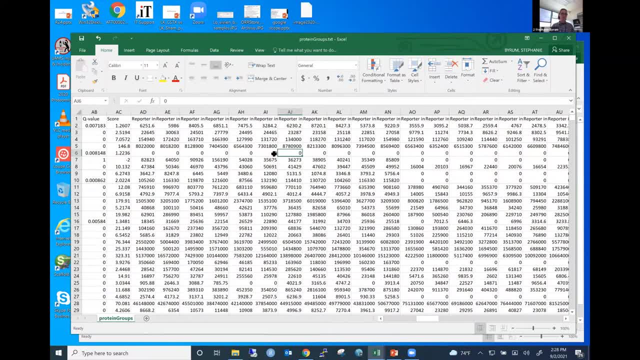 I have a, depending on projects, I can filter to where two thirds of the replicate have to have a value and one of the groups. you can set different levels of filtering to kind of get rid of some of those proteins that don't have that much. you don't have replicate information on. 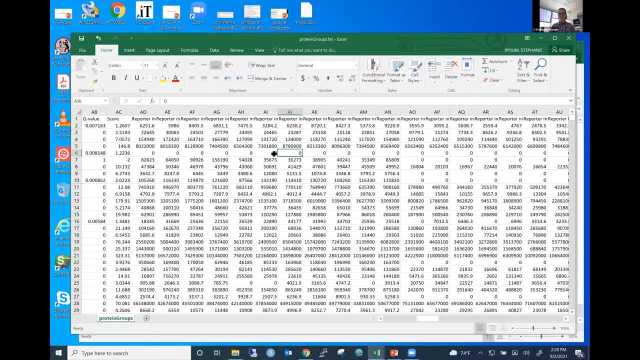 So there are some levels of filtering that you can actually do prior to doing a batch correction. So that particular protein had just enough of an MS spectra to be identified but not enough for a quantitation. But there are some levels of filtering that you can actually do prior to doing any normalization or statistical analysis. 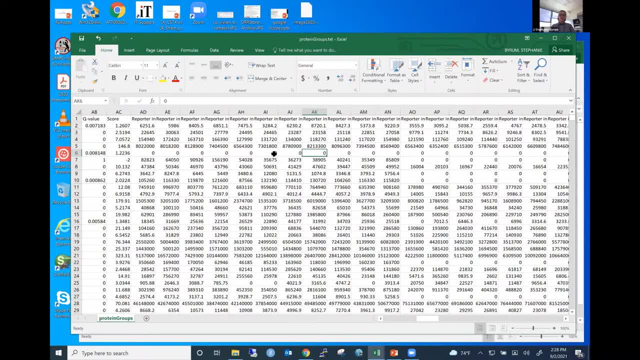 And that can be kind of project dependent. So a lot of times if I'm kind of questioning what to filter, I run it with all of them And then you can look at those GLEMA plots and evaluate a little bit more And then you can do some filtering and rerun it with the removing some of those missing data. 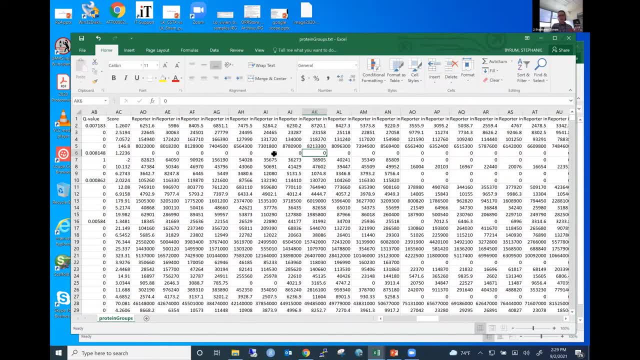 But sometimes those low abundant molecules, proteins, pop out if you don't filter them out, and they can be biologically interesting. And so I try to err on the side of not throwing too much out, because it is discovery phase. but if you're just interested, 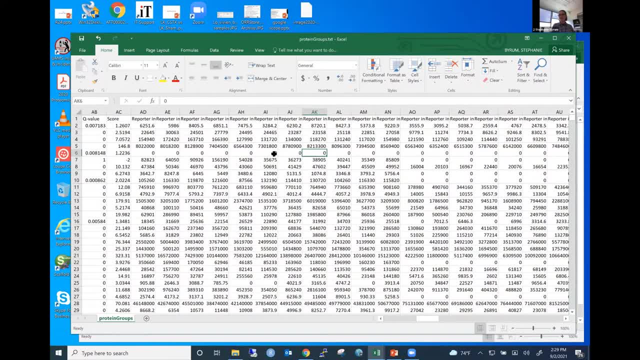 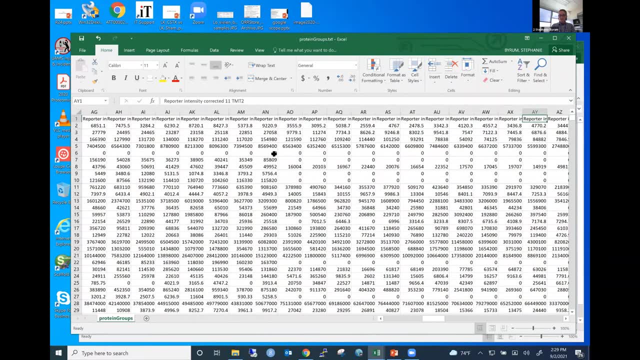 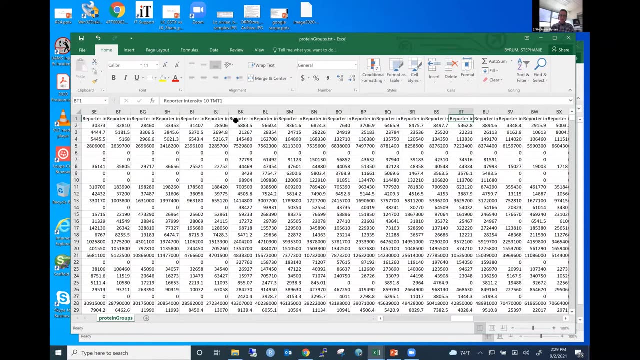 in the top, abundant changes, then you might as well just filter it out. Depends on what your goal is and what you're interested in, But there's, there's, ways of handling all that. So these, if you'll notice they don't have that corrected, So that's going to be the original. 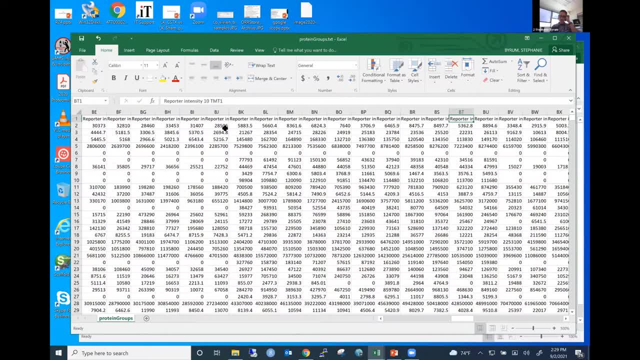 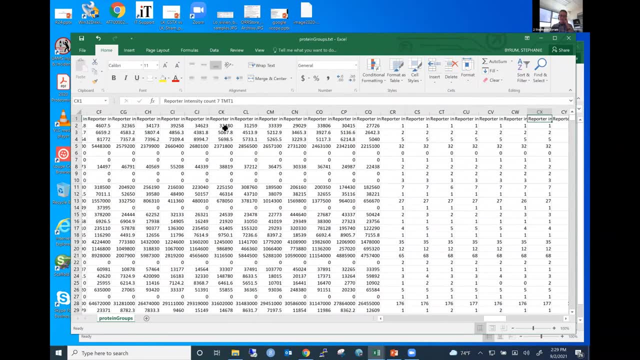 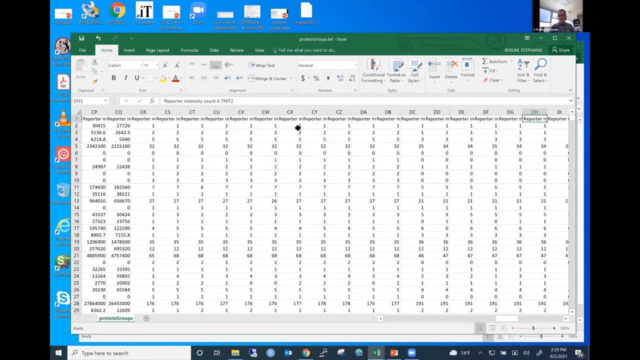 intensity without that reporter ion error correction information. So it does matter which columns you pull out to do the analyses. And then we have the count data, And the count data is the number of MS spectra that we have for each of those proteins. So yeah, zeroes is not really. 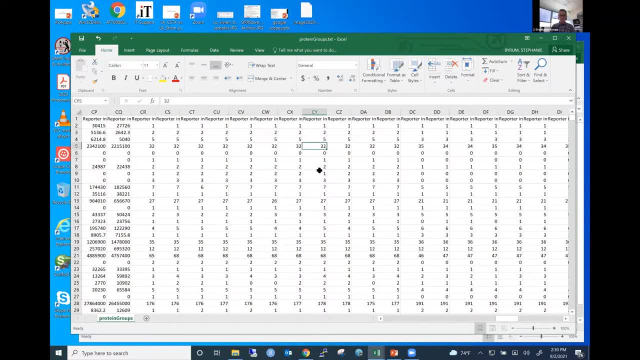 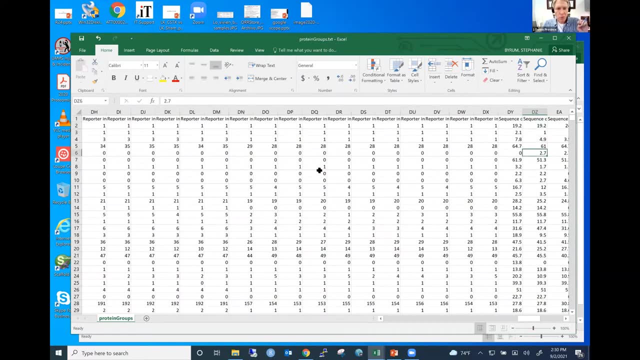 important. So yeah, zeroes is not really important. So yeah, zeroes is not really important. So yeah, there. So that should get removed. Stephanie, can I just ask a question there? So the one that has 34, that would have maybe 34 different peptides that all have those tags. 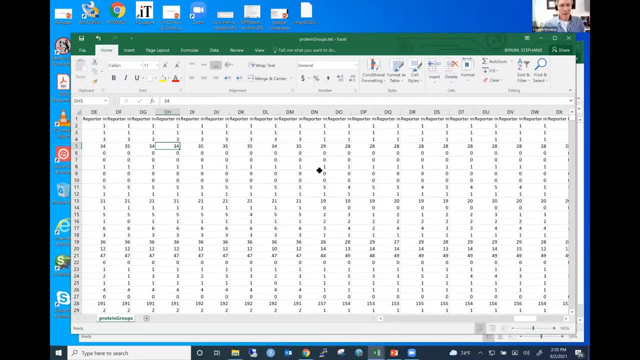 Yeah, MS2 spectra, That corresponds back to that particular protein. Well, the other one maybe just has one. We only found one peptide, So therefore it was only one tag Right, Does that seem OK? Thank you, Yeah, And that's something like a label for your project with count data, like we do. 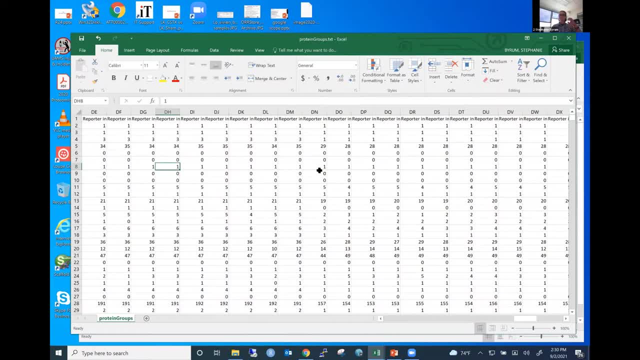 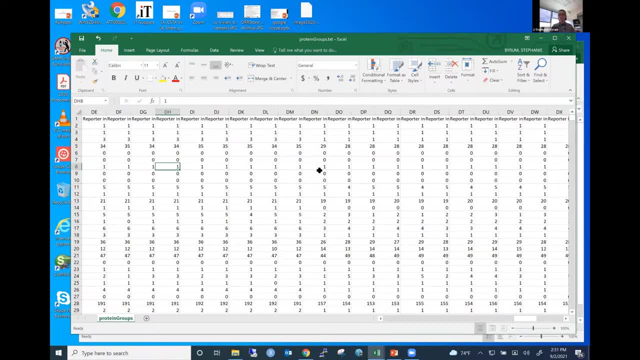 Yeah, So that's something that we would do. Yeah, So that's something that we would do. Level- So you can have some filtering at the count level with label, free type data as well- All sorts of things you can do with data. 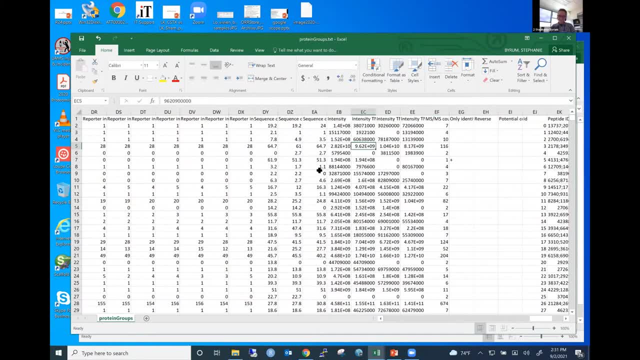 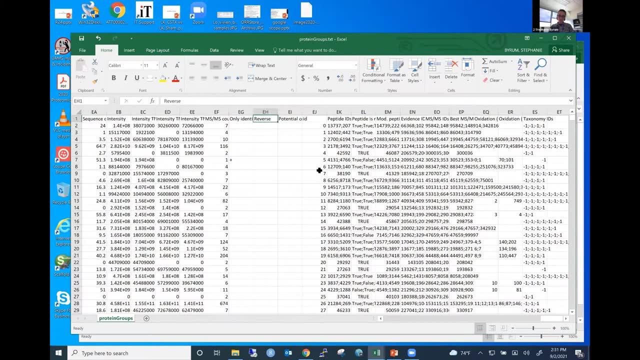 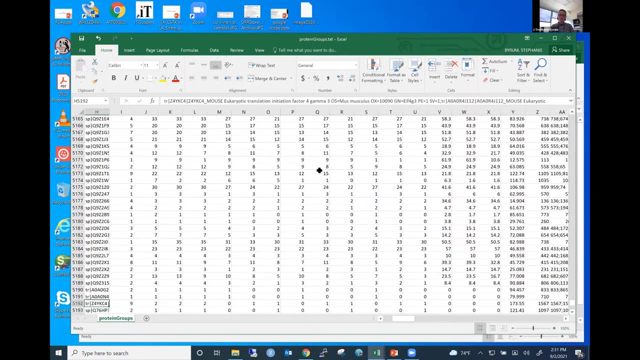 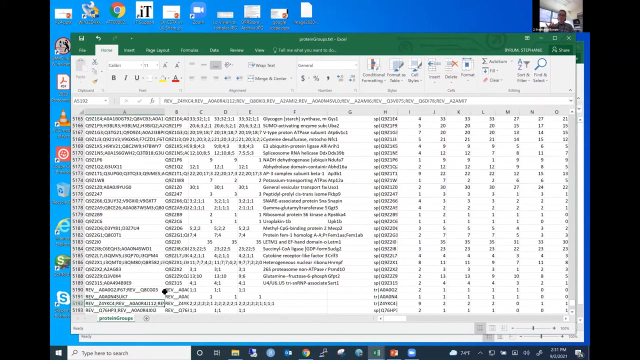 That's what makes it fun, right And challenging. So at the end of this big file we have this reverse and potential contaminant column. These are the ones that are flagging the reverse sequence information. So this has that reverse at the beginning of that label. That means it was matching the reverse sequence of. 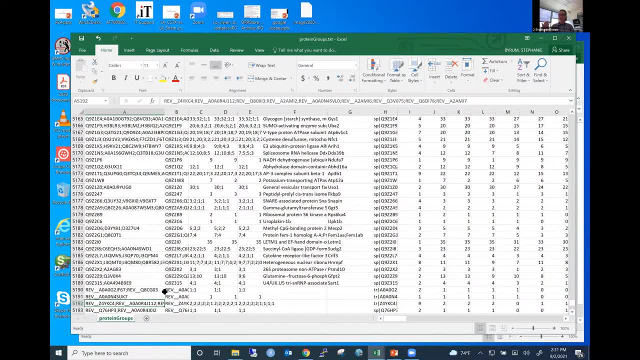 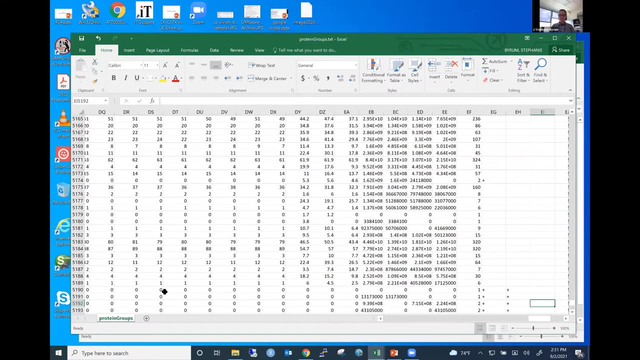 that protein and should be removed. This is how you're calculating a target to decoy ratio for your false discovery identification, And we're trying to set that threshold to 1% for identification error. So that's the reverse. And then we have one that's for contaminants And the contaminant one. these are the proteins That's. 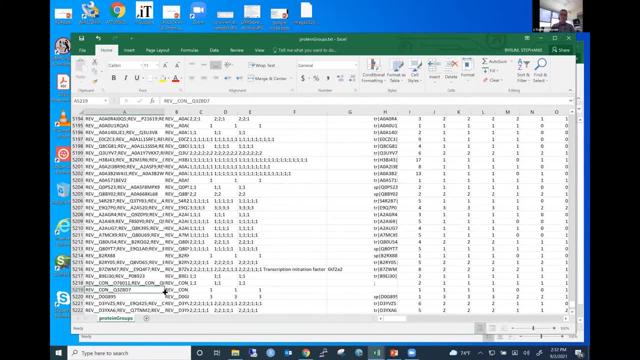 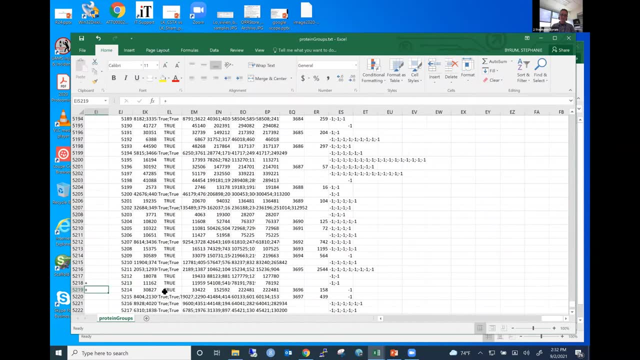 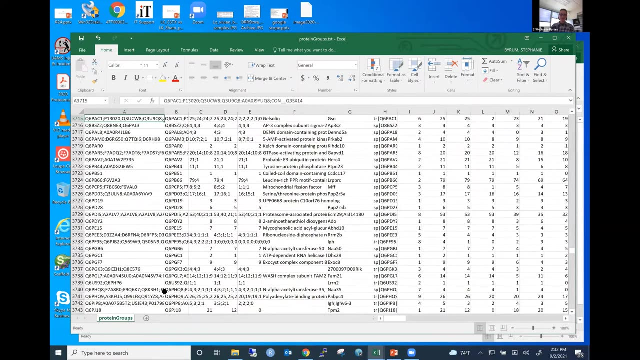 a reverse and a contaminant. So that's even way worse. But the contaminants are the ones associated with the contaminants database. So if I find another one- Not that many in that one- These are my shortcuts. Yeah, And this one, the contaminant is actually that. 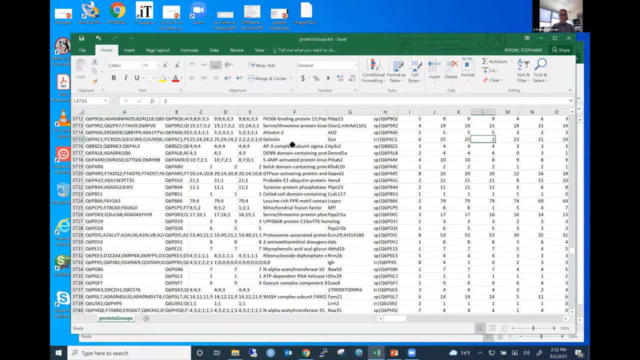 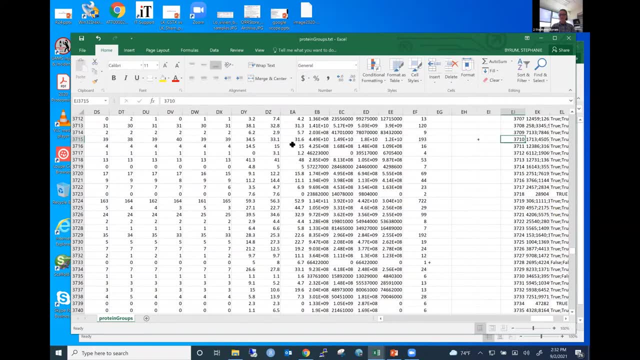 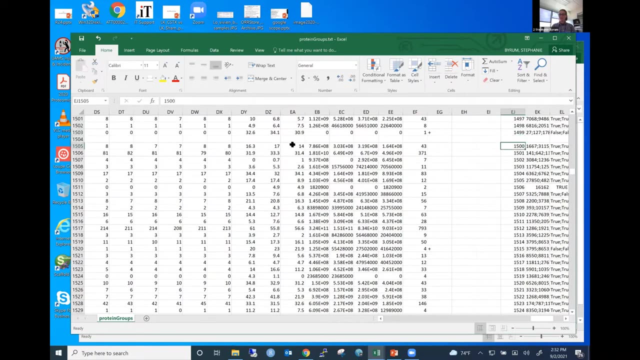 last one in there Just kind of interesting. I've seen some goofy things with max font output files. Sometimes they're not all consistent, Like this right here, And this is like a programmer's nightmare Because it's never a consistent pattern And so you have to kind of find these empty columns in here where it's just a bunch of. 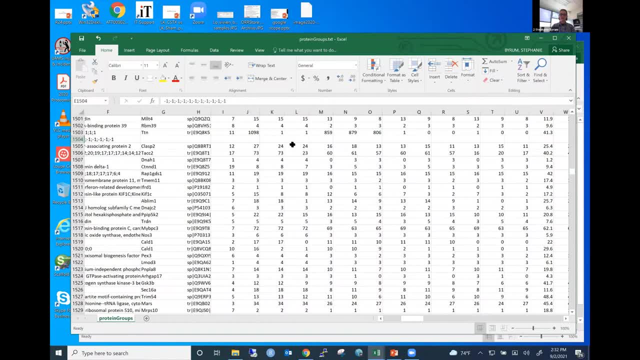 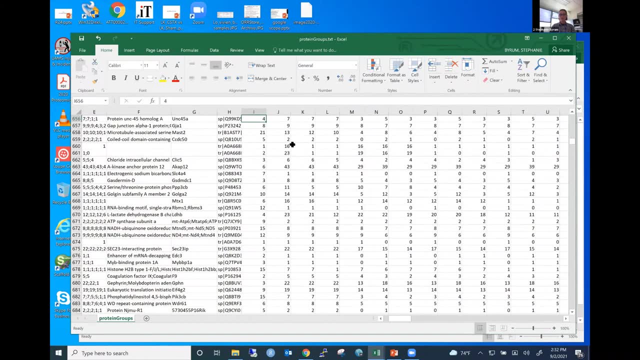 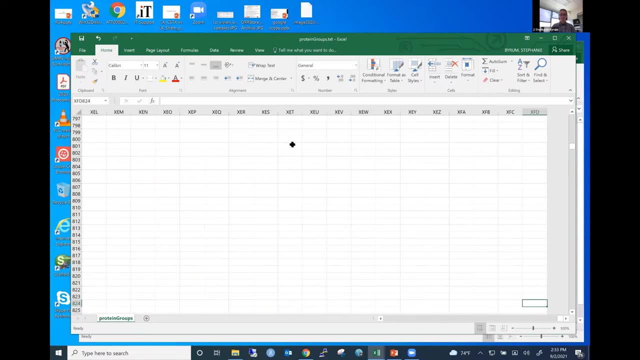 gibberish And they can kind of mess up your data frame. So when we're pulling out information out of this, you may only pull the first few rows and not all of the data, just due to having these kind of extra little miscellaneous identifiers in here. So I have seen that quite a bit too. 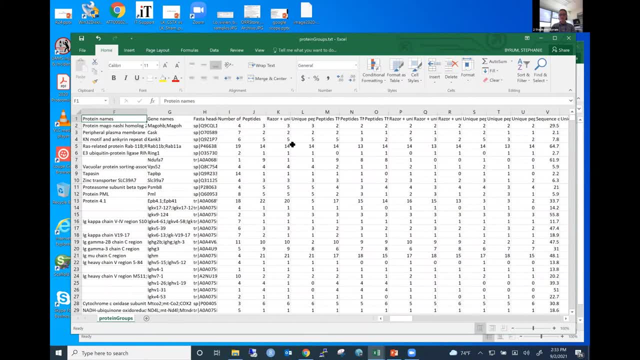 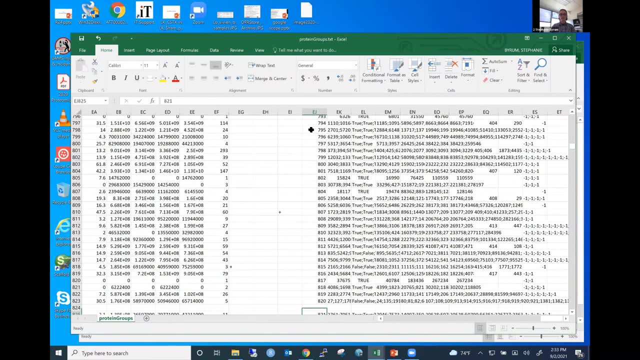 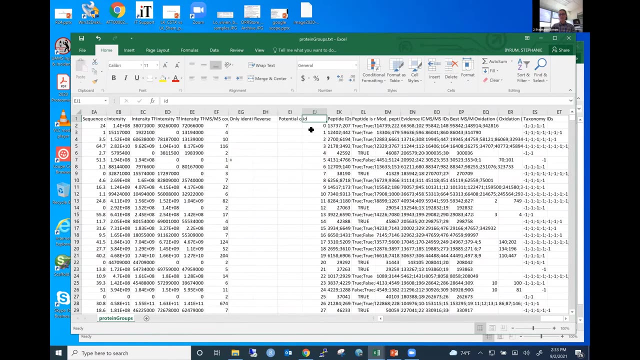 So one way to get around that is actually just sort sort this by this ID column first And then all of those will be at the end and you can get rid of it and stuff. But I'm starting with just max quant output is really painful. It's just. it's kind of a painful learning process. 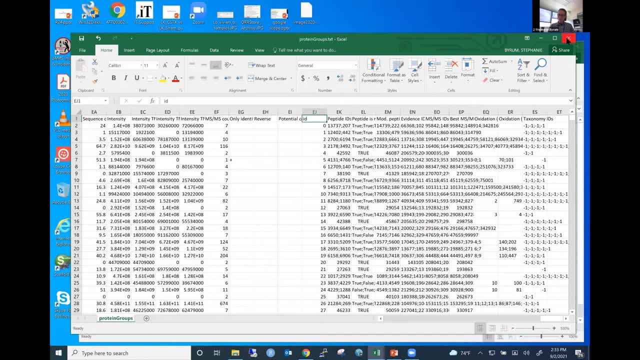 So from the what we would do with the proteomics core, once you submit your samples, it goes through the mass spec, Then the bioinformatics team. we take over and process the data. We do the normalization of all the data sets And then provide the differential. 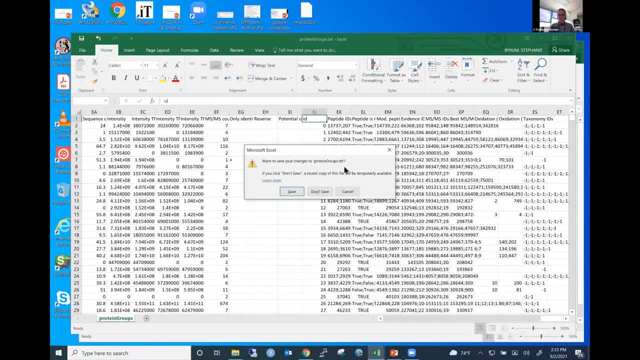 expression analysis at the end. So I'm going to any questions about this file. I'm going to close it. I have another question. Okay, Do you consider any like, like when we talk about RNA-seq data and we're looking at counts? 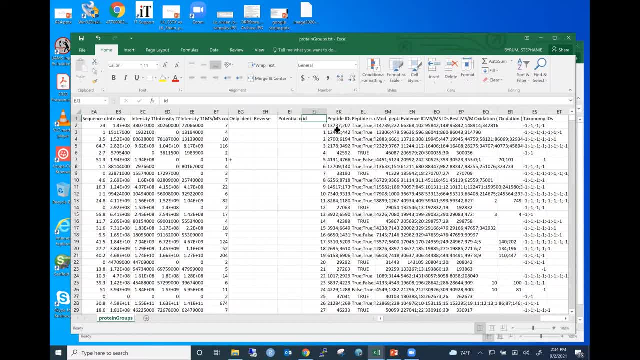 like anything under 10, we kind of in the core, think of it as noise and don't really trust these. If we see two, two, two, two, two, like we'll get rid of that gene, right, Right, In terms of reporter ions, is there a level that you just consider semi-noise? if you see 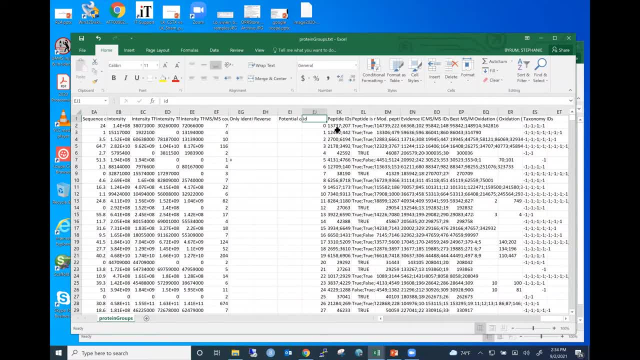 it all the way across. let's say it's a thousand across all of them. It's like: well, this is not a true abundance measure. Do you have a level that you look at or not? really, We don't have that yet for these, for the intensity level, But I kind of utilize. 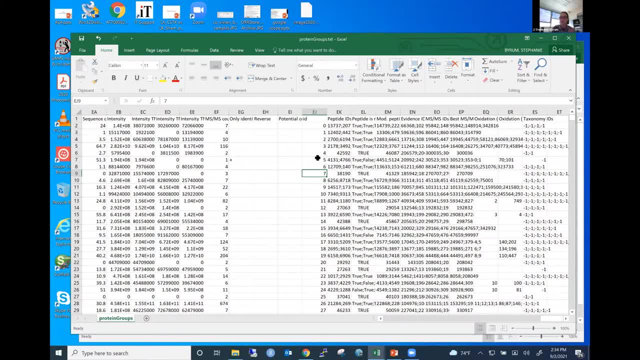 the MD plot to kind of look for those, And then we can set a threshold with that plot if we need to to remove some of those lower abundant ones. But yeah, there's not really a set threshold for filtering on that level yet. Great, Thank you. 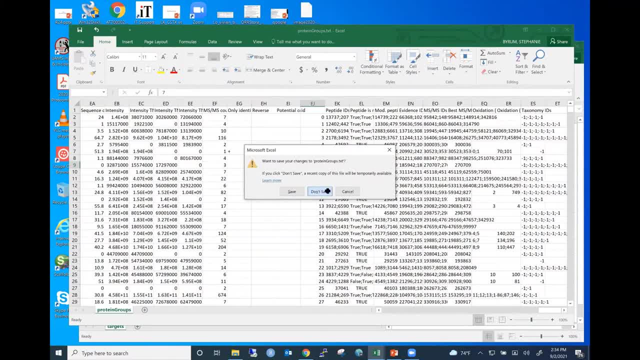 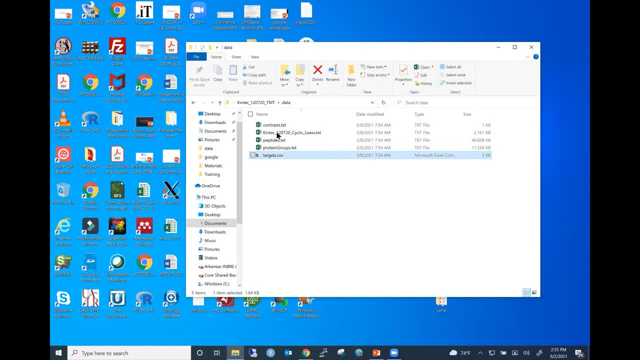 But there should be. I think It's just kind of that abundance issue. Yeah, we don't have one either. I don't really filter on low intensity, So I was just wondering if you guys do. Yeah, no, not yet. 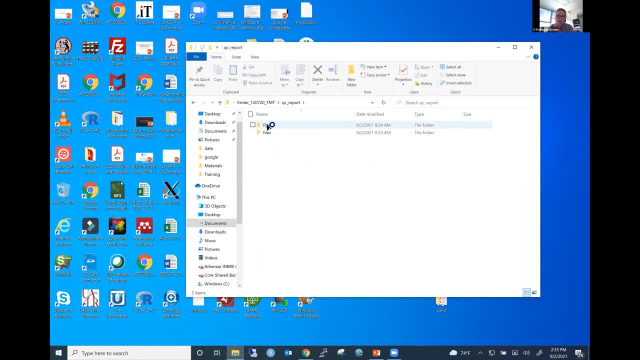 Okay, We already looked at protein norm. I've got some QC figures that we do. It's just the clustering and PCA, So I'm not really going to go over that anymore, But our results file. this is what we would actually provide. 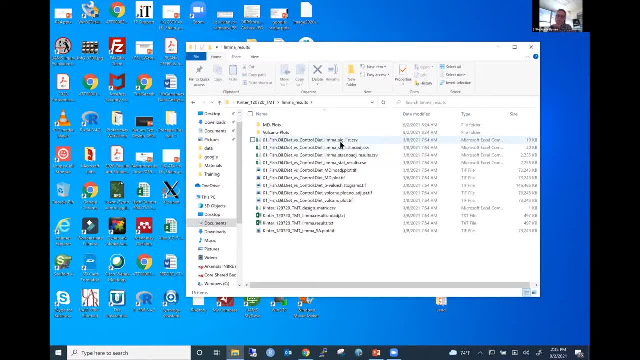 as the results. So we have our significant list at two different levels of significance, whether it's with the unadjusted p-value or the adjusted p-value, And then we have the the full result table, and then static images of the plots, as well as the interactive ones. 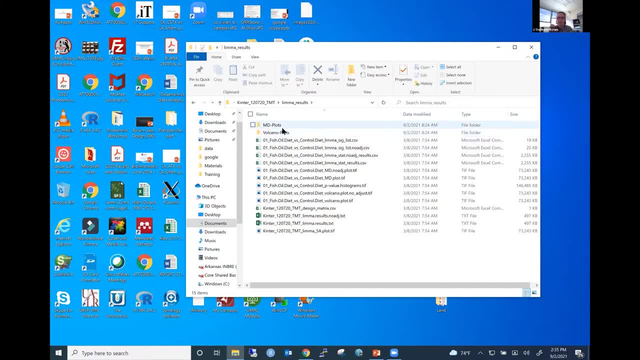 So one thing with these is the interactive plots you'll have to. when we load these into a box folder, we try to zip them to save space. in order for them to open up, you have to extract it and unzip the files. 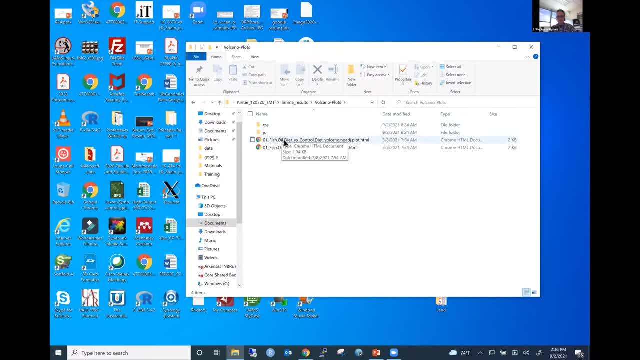 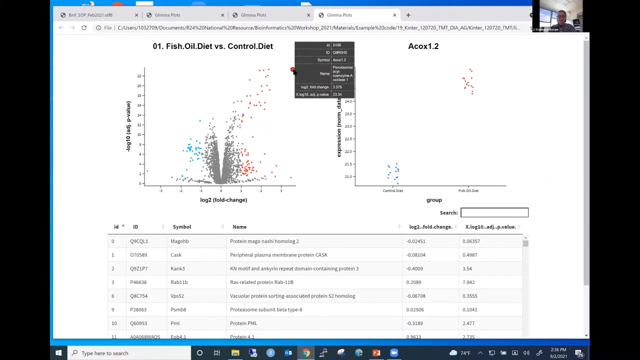 So then, once you have these files, this HTML report is actually pulling the data out of these other two style sheet folders, so that's why it's got to be unzipped, And then you can open it into a Chrome web browser, and now we have our interactive plots. So this is just trying to 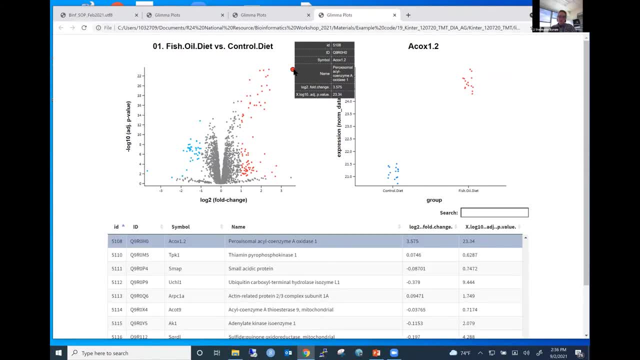 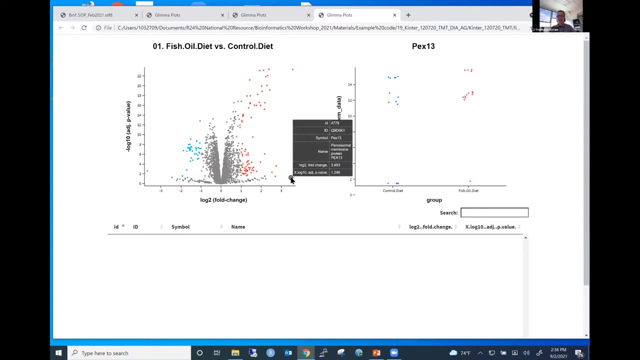 take all of that output and put it into an interactive platform so you can quickly look and see what protein it is, what p-values are, and then connect it to the normalized intensity values And because, a while ago, this is really a tool that I use a lot to kind of. 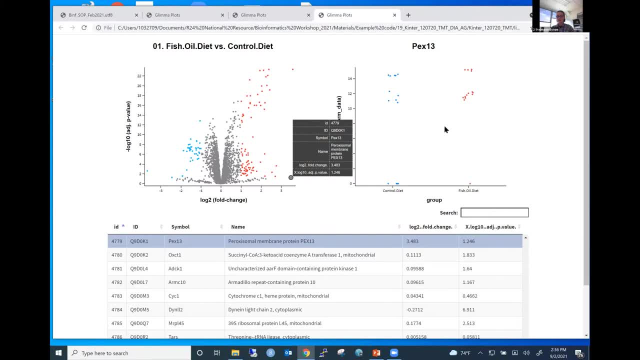 look for things like this, where you have a missing value or not. One thing on this analysis: we're displaying the missing values as a zero in this plot, but it doesn't mean it was a zero in the analysis. There's one thing that you have to watch out for with the LIMA. 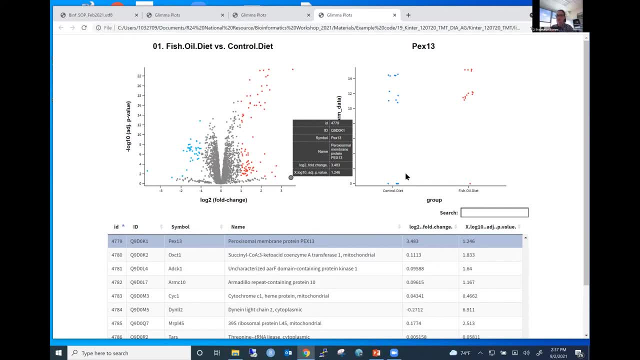 when you're doing an LMFIT model design. If you have your missing values set as an N-A instead of a zero, then any protein that has the N-A is emitted from the statistical analysis. If it's a zero, it's included and will impact your fold change. So it depends on how you set that those 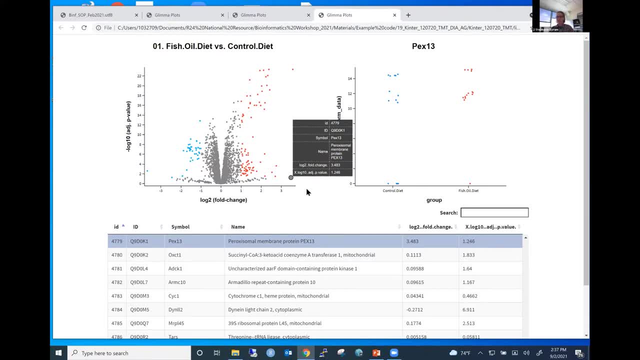 missing values before you do the statistics kind of how it's going to impact your fold change information. So I have found that kind of little caveat. Sometimes with IP experiments I kind of have included it as a zero because it's more of a present absence kind of analysis You're. 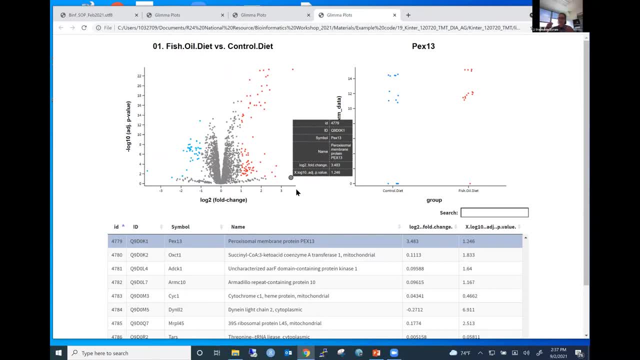 looking for what was in my background, subtracting those proteins that bound to a background beads versus what. So that's kind of what comes down in my actual antibody target. So I kind of have to think about the analysis a little bit differently with IP experiments. But yeah, we would provide all of 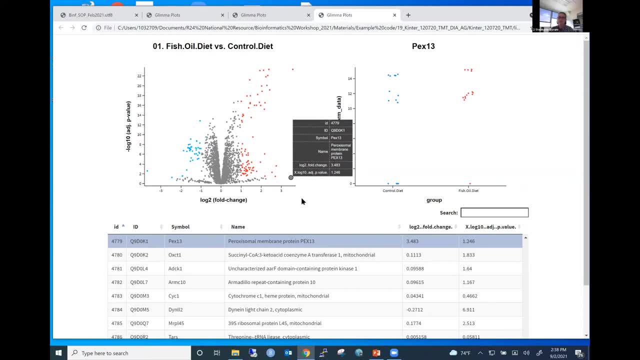 this data for the end results. zip all that up, give it to the end user along with the scaffold file, all of the raw MaxQuant output, so then you can do any type of analyses And ultimately, what we'd like to be able to do. 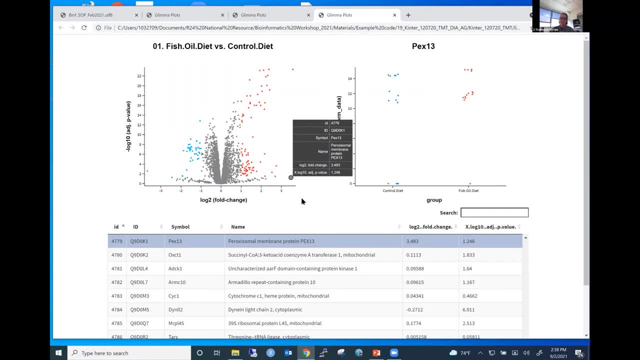 is partner with the idea states, So whenever a user comes from a particular state, we can connect them to one of the other bioinformaticians that can help with the downstream processing of pathway analyses and any of the extra analyses that they want to get. 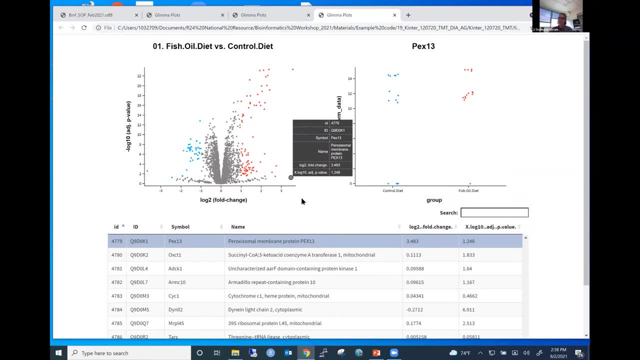 to a publication. So I'm really hoping we can utilize this network to kind of provide that resource to help one another out and help our end users get to publications. So I would love to have that happen because there's a lot of data to look at. 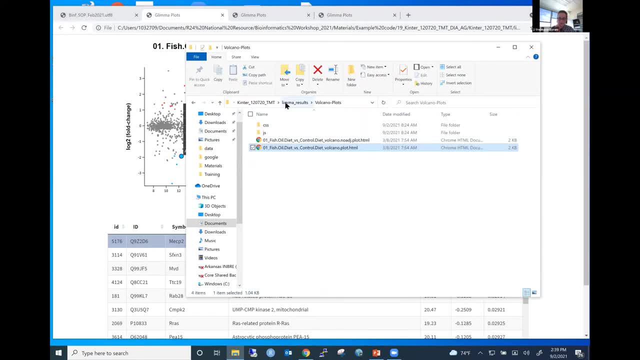 Alrighty, so all of those results would be sent to the end user. We do try to make- and I don't think I have it in that one, I think I made it in this other example And it may be actually in this one. Like I said, I got a lot of stuff. 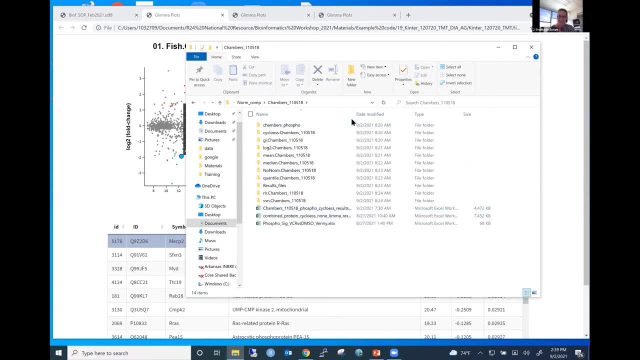 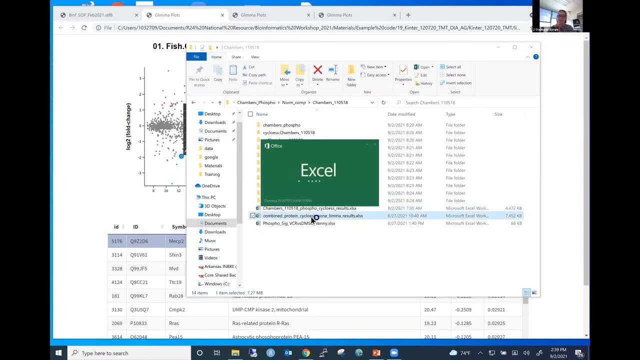 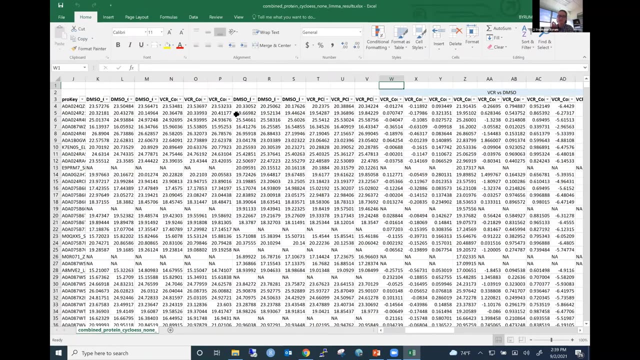 So try to make a simple kind of Excel results file at the end of the project. that's going to contain most of the data needed for making heat maps. any other statistics, like any other plots that people need for publication, get to their significant list. 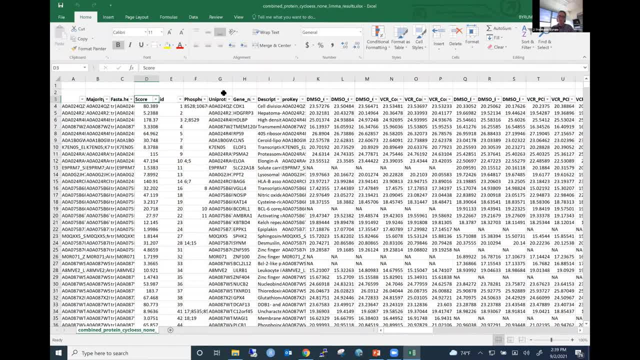 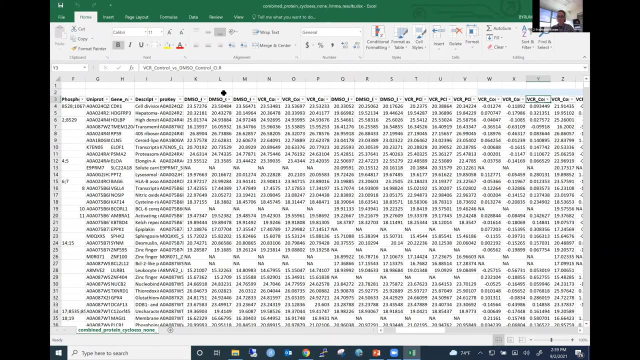 So we tend to kind of make like a more Excel friendly version of all the output. that will have the headers up here what these columns represent, which I haven't done on this one. But these are each of the individual samples from this TMT experiment and 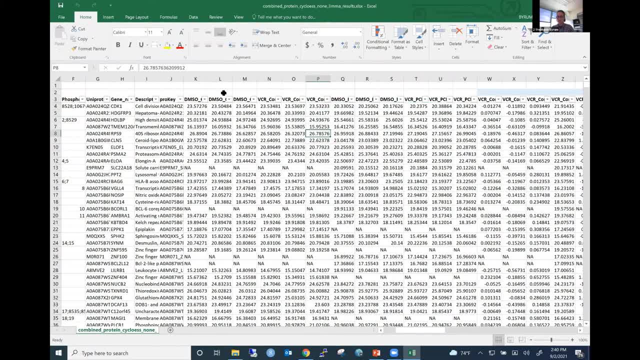 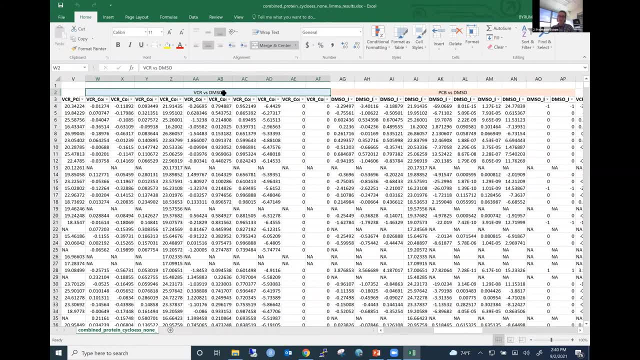 their normalized intensity values And you can see where the NA's are. And then, next to those, are the each of the different comparisons that we did for the statistical comparisons, along with the output from LEMA. So one thing to note on the LEMA analysis. 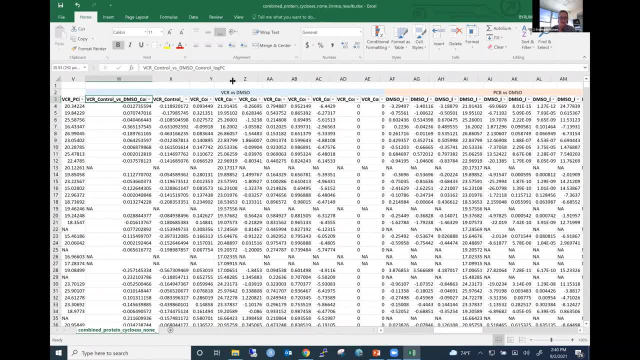 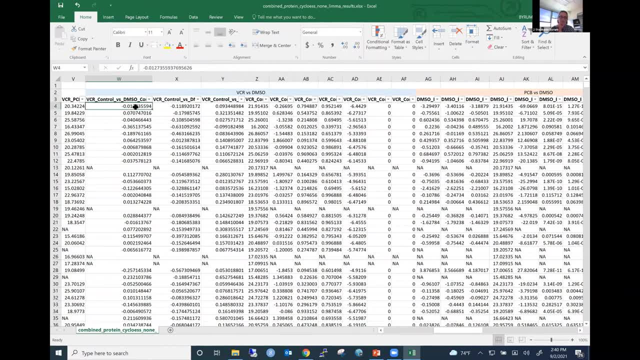 so we have the full change information is log two scale. It comes out as just log fc, but it's a log two scale full change information, followed by the confidence interval, the left and right confidence intervals of that full change information, And then you have the average. 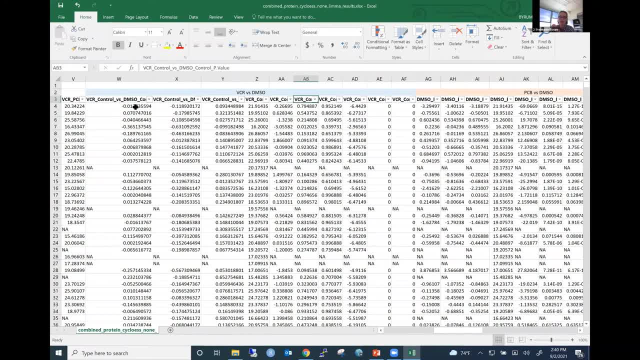 expression versus the t-statistic- unadjusted p-value and the adjusted p-value, along with the b-statistic, which is the log odds ratio. The added columns that we've included also include this sig p-value or significant FDR, And what these are flagging are the ones that are significant by both a p-value and a. 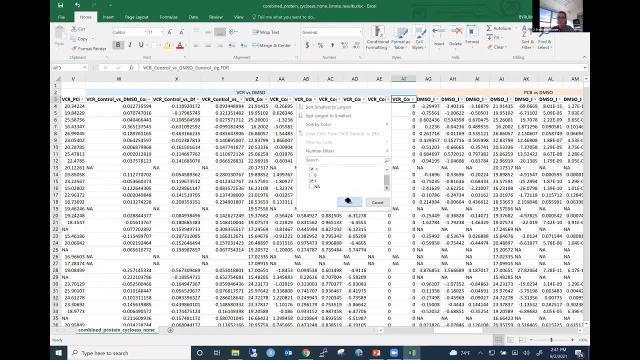 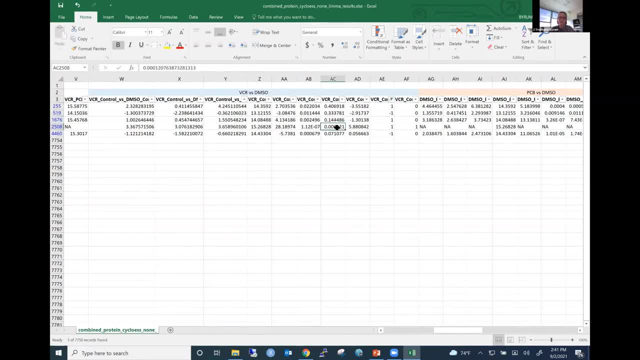 full change. So you can quickly kind of filter through here to get to my significant list at this unadjusted p-value level in the samples. So just the way of looking at it, I'm filtering through the data with two different metrics of significance. 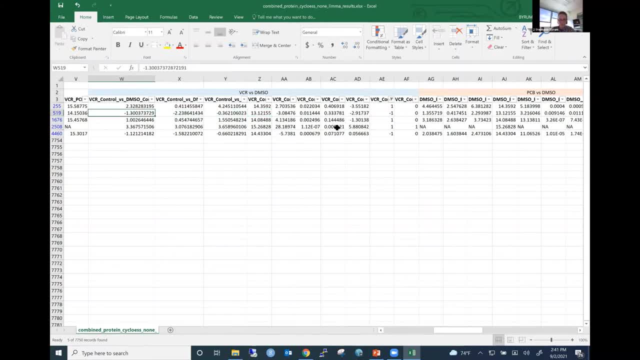 more stringent threshold With the confidence intervals. if that full change happens to have a confidence interval that is on the same direction, either both positive or both negative- then you're going to have a significant unadjusted p-value. Because this unadjusted p-value here is 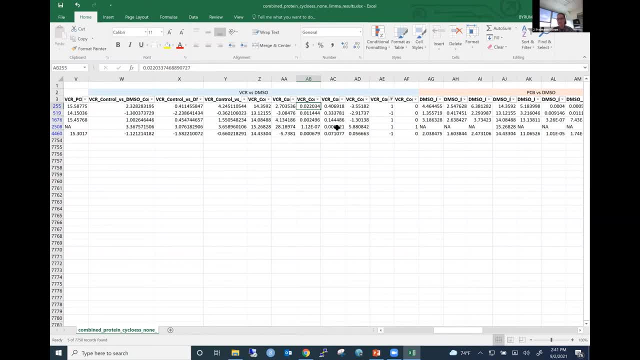 taking into account the standard error of the full change information. So it already does kind of calculate some of the full change information within the unadjusted p-value quantitation. So when I'm trying to do like a pathway type analysis, I'll tend to expand out the 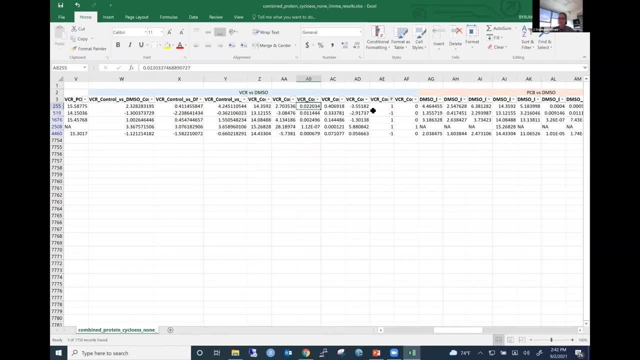 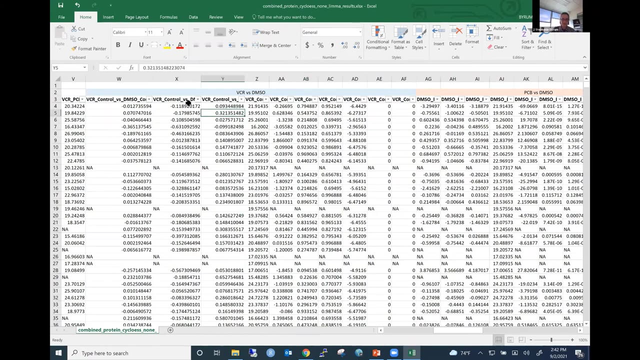 significance to include anything with the unadjusted p-value significant and not the more stringent cutoff, if that makes sense. Because for the pathway I'm trying to kind of include more molecules in order to do a better pathway type analysis. But it is interesting to kind of look at your changes of full change information compared to the 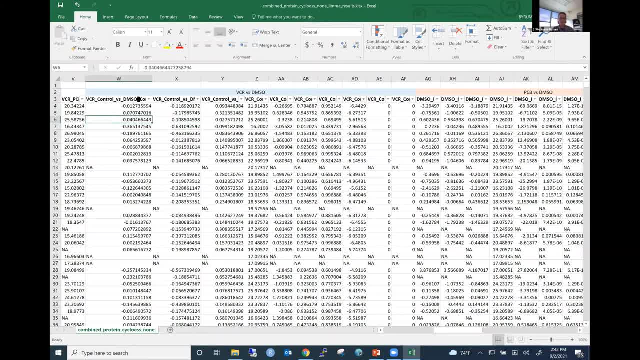 confidence intervals. So, like this particular one, it goes across a zero, you have a negative and you have a positive value, So that, one, your unadjusted p-value is actually not significant And it's reflective of that, So that one, your unadjusted p-value is actually not significant. 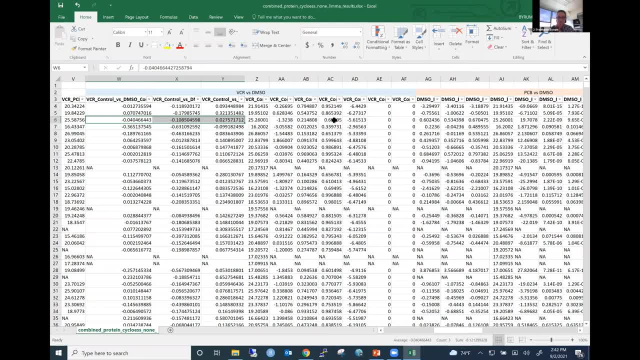 And it's reflective of that, That confidence interval. So we do try to kind of give people a list of here's your top significant proteins that we have confidence in, and kind of that more stringent list to start with. Does anybody have questions about that? 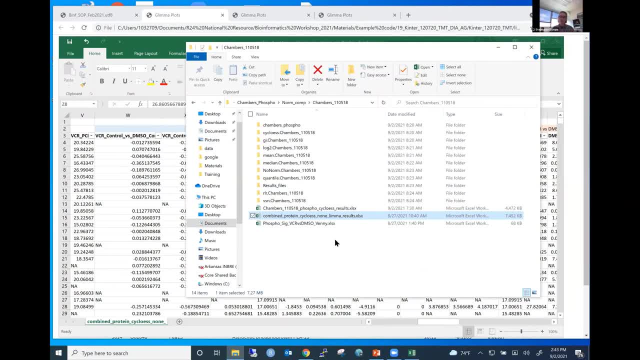 So when we go through this full analysis, we'll run the pretty norm, we'll kind of give like the metrics of what the methods look like, we'll tell you which ones were used and provide all of those differential abundance results, And then from there is where the real fun begins and people have to. 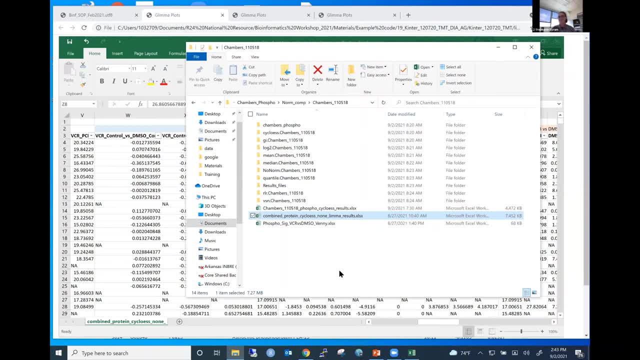 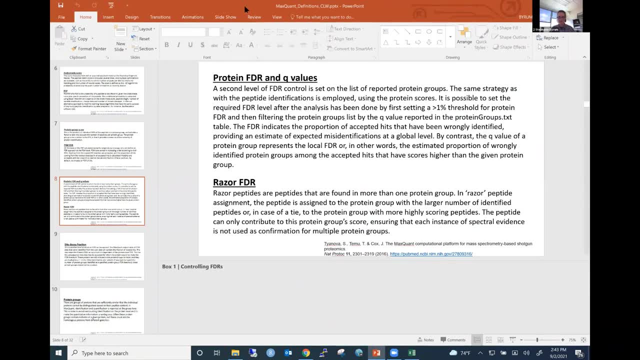 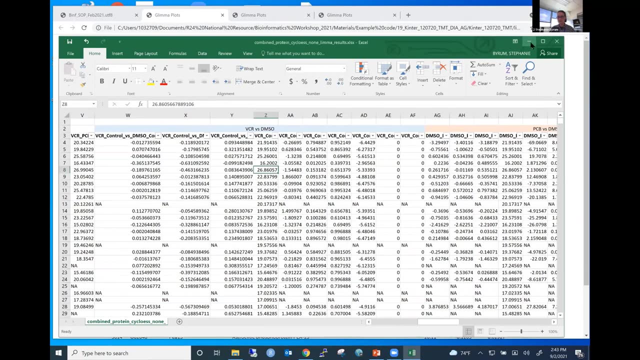 that's where you have to dig into the biology and figure out. what does this mean? Okay, yeah, these are my definitions. I'll send to y'all in the Slack. We got that. we got that. I think we are about ready for our discussion section. Okay.